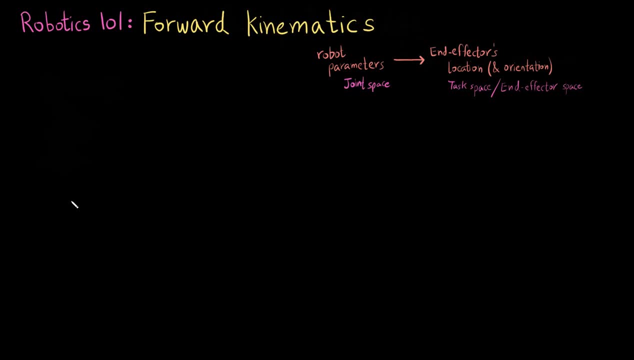 or the end effector space. So what is the joint space? It is the space in which you have the robot parameters defined. So if I have a 3R robot, it is going to be the three angles of the revenue, joint and the end effector space, or the task space is basically the location and orientation of 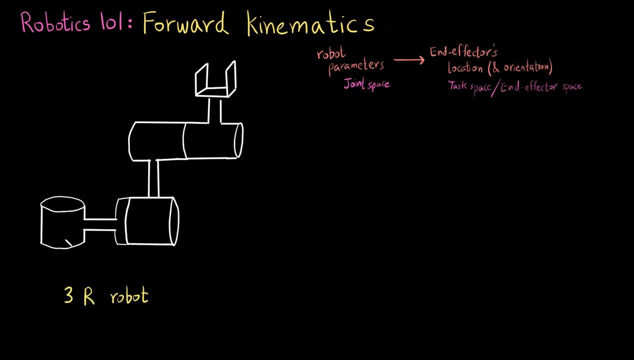 the end effector. Here I have a 3R robot which has three revenue joints, so it is a three degree of freedom robot. This is the kind of robot that you can expect to see in an industry where the application is such that there are two conveyor belts and you need to pick. 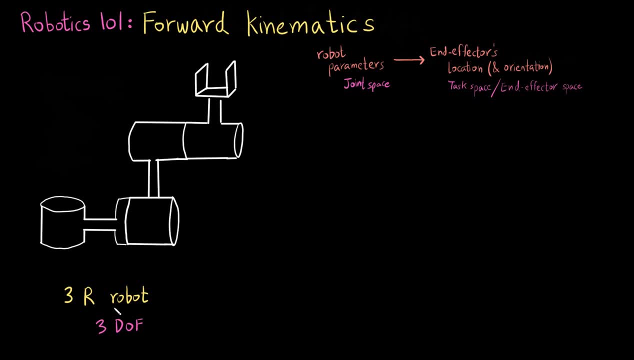 and move objects from one conveyor belt to the other. So in the very simplest of cases you might be able to see this kind of a robot. So it is a 3R robot. so here I have marked out the rotation angles. so theta one is the rotation about this axis. theta two is the rotation about this axis. 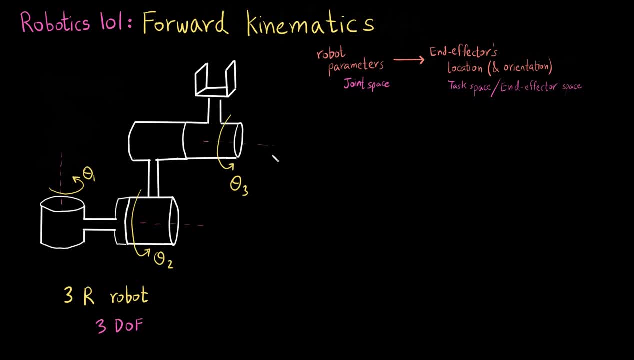 and theta three is the rotation about this axis. Now, since we are doing forward kinematics, what would be provided to us would be the exact values of theta one, theta two and theta three, and we need to figure out where the end effector would be based on those specific. 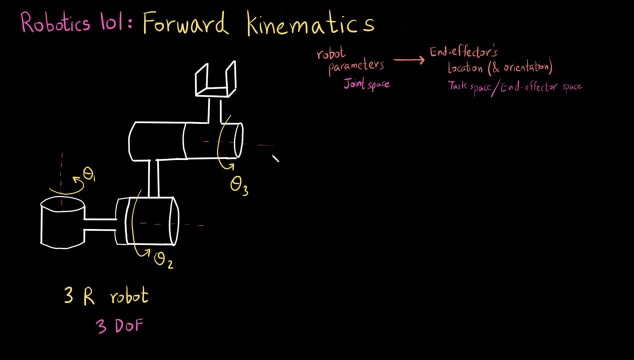 values of theta. So, in order to figure that out, first what we need to do is we need to define the fixed frame and the moving frame and, as always, what we do is we define the fixed frame to be at the base of the robot. This is the fixed frame and the moving frame of the robot, And then you need to 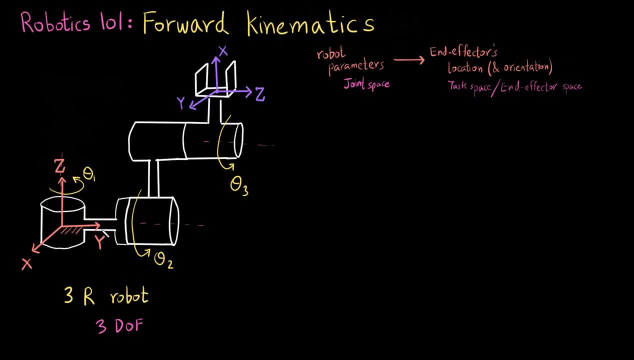 normally what we do. however, that isn't that there isn't a composition for us to do it this way and we can keep the fixed frame to be at any point in space. it can be at the edge of the room or at on one side of the conveyor belt or anything, so it doesn't really matter where the fixed frame is. 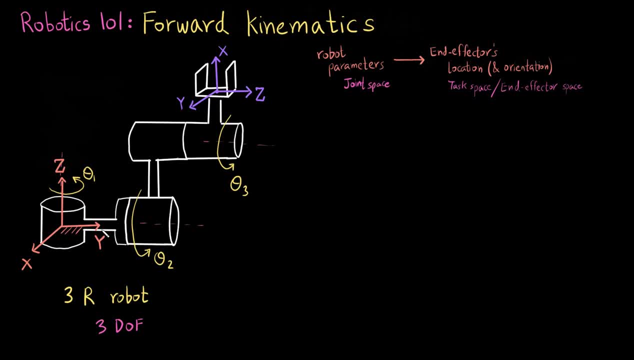 you just need to have all the other frames defined with respect to the fixed frame, and the moving frame is defined at the tip of the end effector. so here i have to find it right here. so it is a gripper, so i have defined it at the base of the gripper. so this is my moving frame. 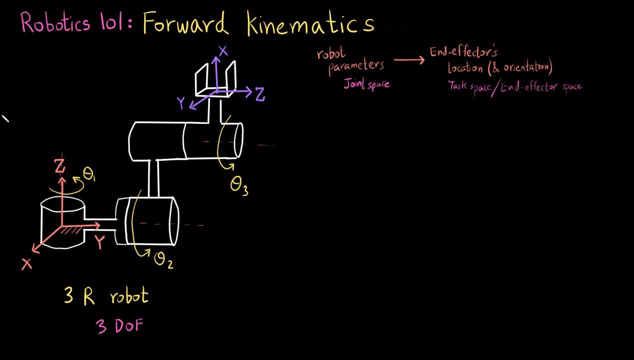 and now what i need to find out is a homogeneous transformation matrix that takes the fixed frame to the end effector frame. and if i find out that homogeneous transformation matrix, then i should be able to extract the displacement vector out of it, which would give me the location of the end effector. 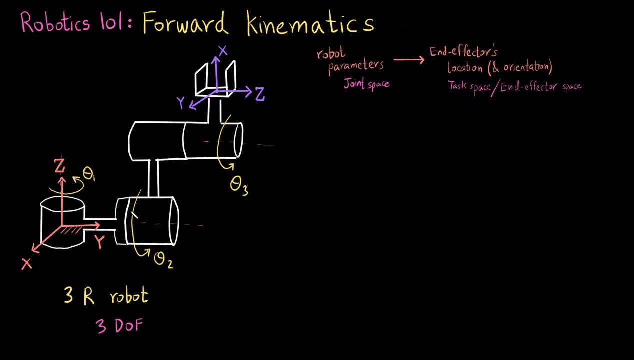 with respect to the fixed frame. so if you have a robot with you, you would know the physical parameters of the robot which i have marked here, which are just the four lengths: a1, a2, a3 and a4. and what we are interested in finding is, again, the homogeneous transform which takes the fixed frame. 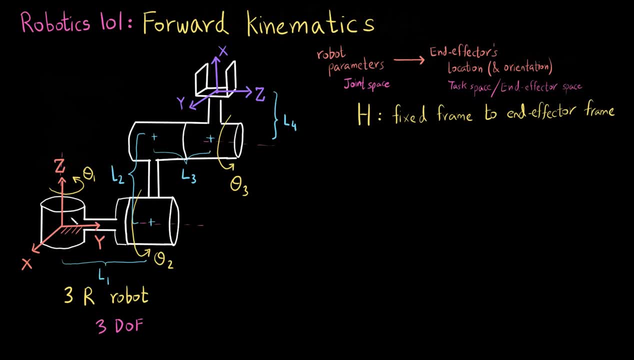 to the end effector frame and, if i draw it out here, so it takes this frame and it takes it all the way to this point right here. so this is what we are concerned with, right. so it takes this frame and it takes it all the way to the moving frame. 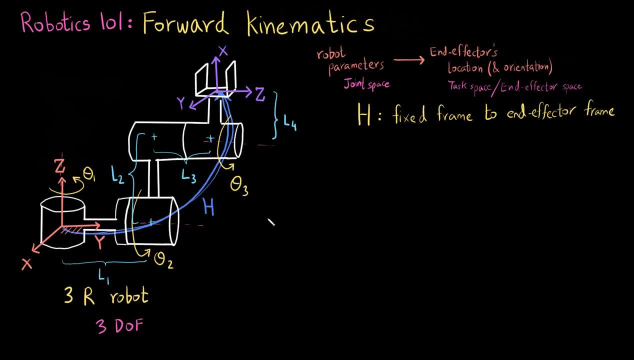 now, how do we find out this homogeneous transform? as we have done in the previous video, what we do is we break this homogeneous transform into a number of steps. so we break this home single homogeneous transform into a bunch of different homogeneous transforms and we multiply them out together. 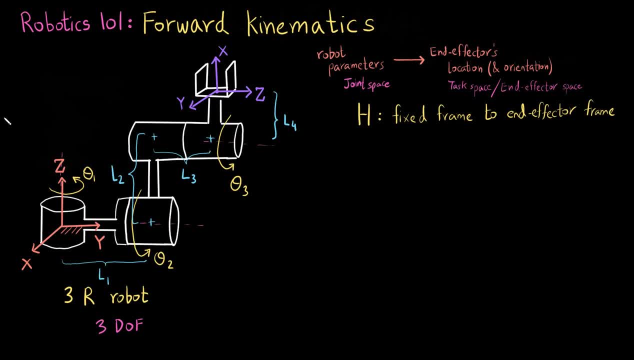 so one way- notice that i'm saying one way, because you can approach this in many, several ways- so one way is to first do a homogeneous transform that takes the fixed frame and takes it to this point, and then it takes this point to this, and then it takes this to this, and then it takes this to this. 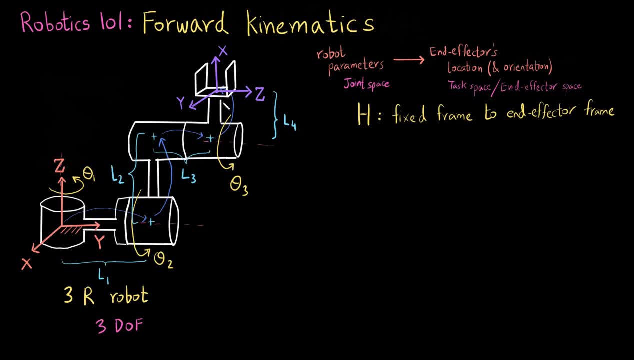 however, on using this end point, which is an effector, you would realize that your frame is not going to align with this right, because once you do either homogeneous transform and you get to this end point, your x-axis is going to be in this manner. however, in 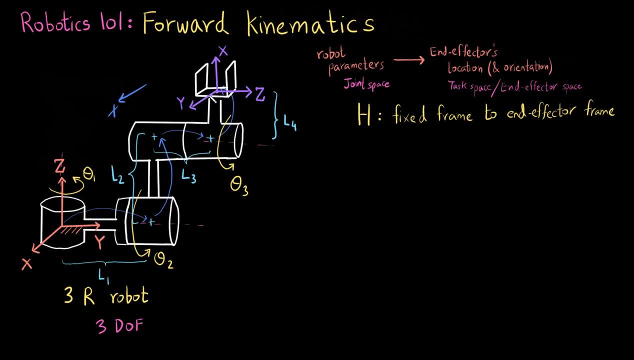 the given diagram, there's y-axis in this direction. so you would need to do another homogeneous transform which just has a rotation matrix inside of it and no displacement, and it rotates it such that my orientation becomes as desired. so notice that I said that this is just one way of doing the homogeneous. 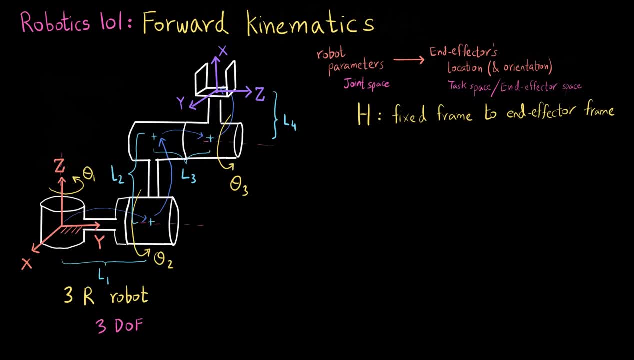 transformations right, so you can approach it in a number of ways. so so you can do it in this manner. so in this, what I've done is there's h1, h2, h3, h4 and h5. so what I would do is I would first do h1. 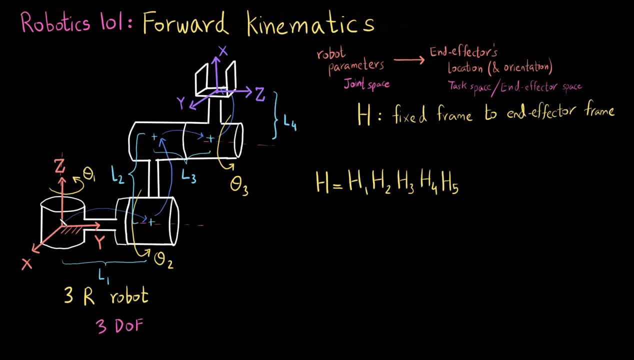 which is the homogenous transform. and then I would do the homogenous transform, which is going to be simply a rotation about the z-axis and no displacement. so the first: your h1 is going to not take this fixed frame anywhere, it is just going to keep it here, but it is just going to rotate it. then h2 is going to. 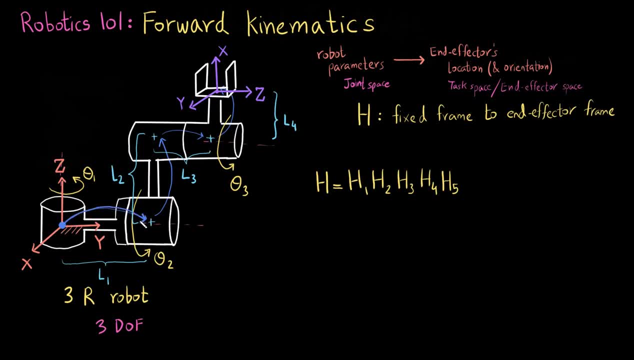 displace it and bring it right here and then rotate it. h3 is going to just displace it with no rotation, h4 is going to displace it and rotate it, and then h5 is going to rotate it and displace it and rotate it as well, and there are a number of different ways you can. 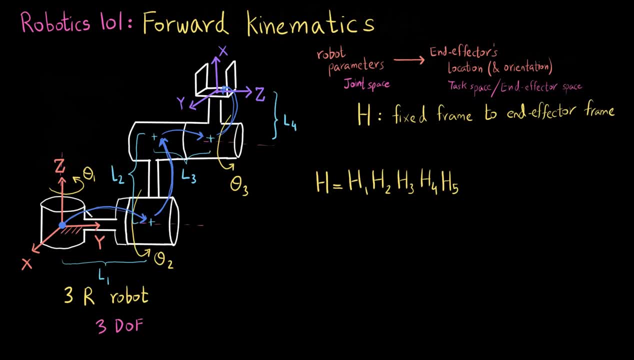 approach this. so another way that you might want to approach it is, instead of just doing the first homogeneous transform, which just has a rotation without displacement, you can just combine the two and you can just call this to be h1. so first you displace and then rotate, and then you can proceed in. 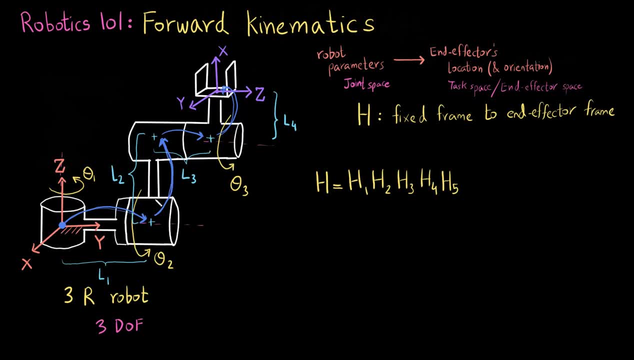 that manner. I hope you get the idea of how to do it. so I would encourage you to pause the video right now and try and find out what you think about it, and I will see you in the next video giving giving it a try and see if you can make some progress into it and then 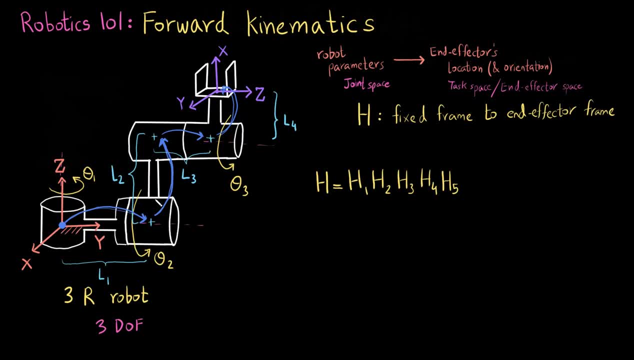 you can play this video and see my solution of it. I hope that you did give it a try, so let me show you my solution of it, the way that I would approach it. so here I have expanded all of these five homogeneous transforms. so my h1 is: 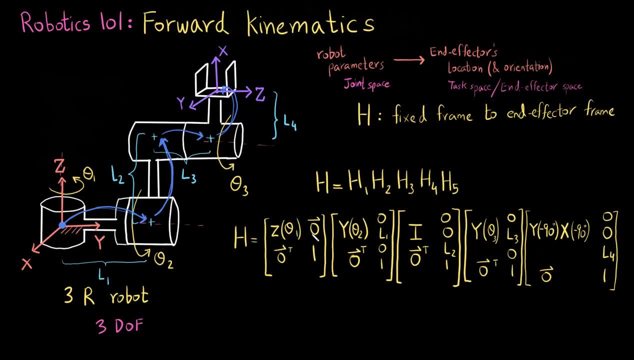 going to be just a rotation about the axis by theta 1, no displacement, and then I will show you how to do it in the next video. my h2 is going to be a displacement by this vector, but just takes it from here to here and then it rotates it by about the y axis by theta 2, and then I have. 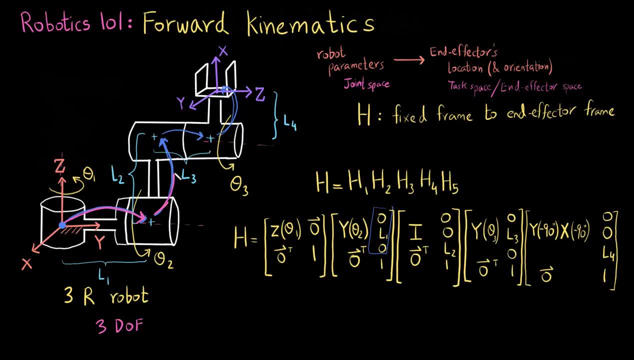 another rotation, I'm sorry, another homogeneous transform which just displaces it from here to where and there's no rotation involved. so you can see that there is no rotation. so I have an identity matrix here and my identity matrix would simply be 1 0 0, 0, 1, 0 and 0 0 1, so it is a 3 cross 3. 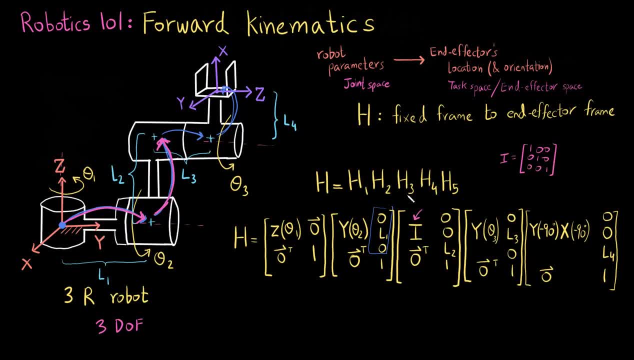 matrix. so so my h3 is going to be this, which is just a displacement, with no rotation. now my h4 is going to be a displacement and then a rotation, and so h4 is going to take it from here to here and then rotate it, and then there's going to be my h5, which is first going to displace it. 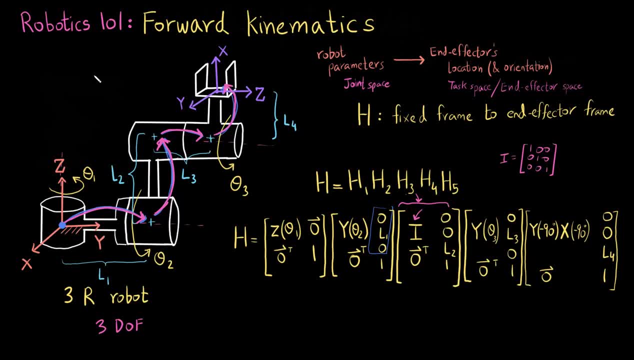 right once it displaces it. so my frame is going to be in this manner: x, y and z. however, you see that the my required orientation is this. so, in order to do it, what i would do is i would first rotate it about the y-axis minus 90 degrees. 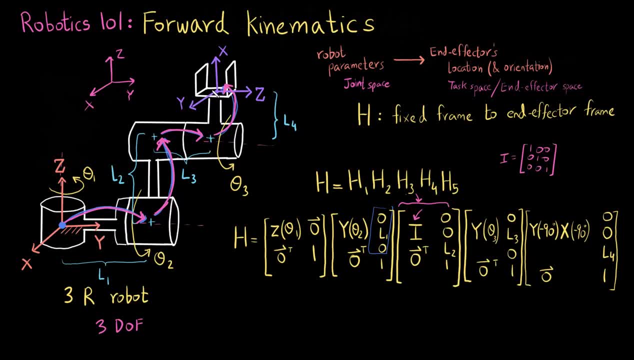 and remember that positive, positive rotation is counterclockwise and negative is clockwise, so negative, uh, 90 degrees. what that would do is- let me draw it out- what that would do is it would, uh, it would bring my x-axis here and my z-axis at the back and my y-axis would remain where it is. 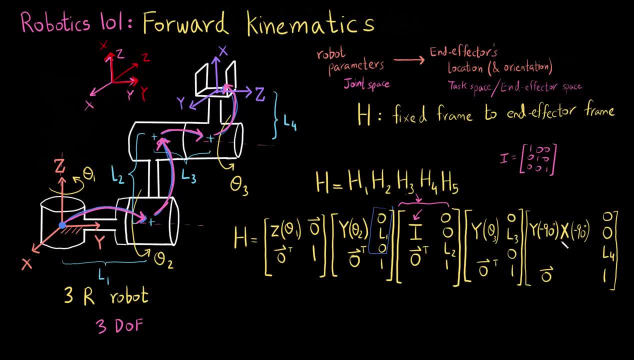 and then what i would do is i would rotate it about the y-axis minus 90 degrees, and then what i would do is i would do a rotation about the x-axis by minus 90 degrees to a clockwise rotation about the x-axis, and that would, uh, make me get to the required orientation. 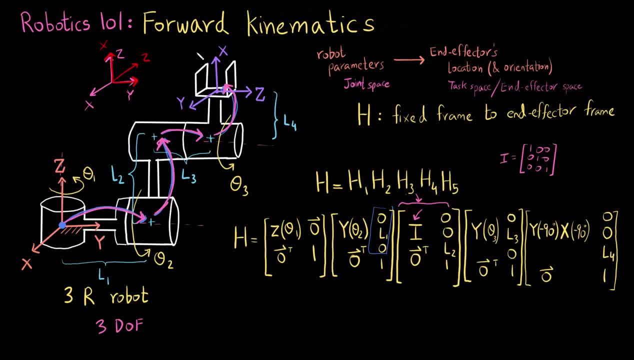 and that isn't the only way to get this required orientation. instead of this, i can do, uh take another approach. so maybe one of the other approaches that i can take is i can do a rotation about the x-axis by minus 90 degrees to a clockwise rotation. 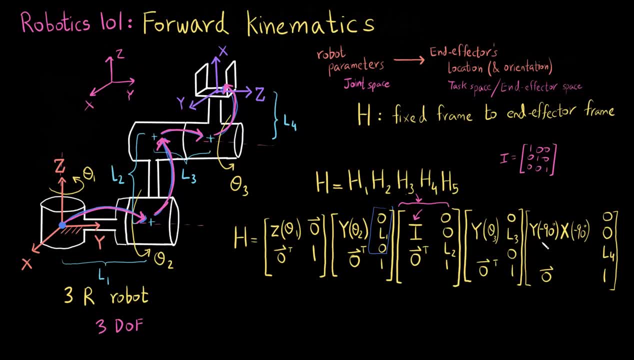 is, instead of doing y by minus 90 degrees first, um, what i can do is, um, i can first uh rotate by x by minus 90 degrees. so if i do that, so what that would mean is my x remains here and my z-axis becomes here and my y-axis goes down here. so now you see that my z-axis is aligned with the. 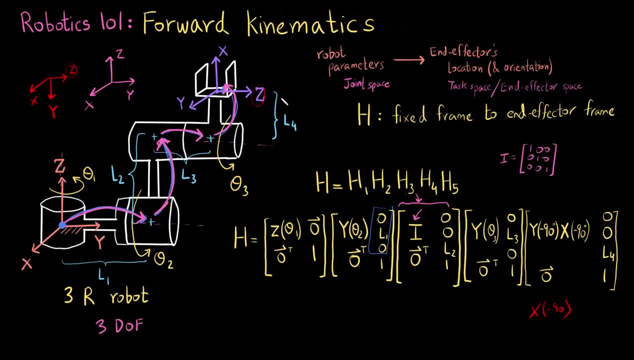 directional z-axis that i wanted to, and now i can do a rotation about the y-axis to a clockwise rotation. i can do a rotation about the z-axis, so i can do a rotation about the z-axis by minus 90 degrees, and if i do that, so, uh, if i do that, uh, what i would get is basically my y-axis would become here: 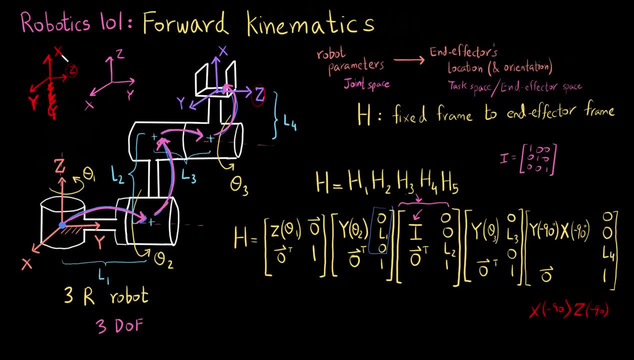 and my x-axis goes up here, and that is what we want, right? so you get an idea that the homogenous transformations, the way that you get to the homogeneous homogeneous transformation, is not unique. however. however, the final homogeneous transformation that you are going to get, which is this one right here, the final homogeneous transformation that you are going to get. 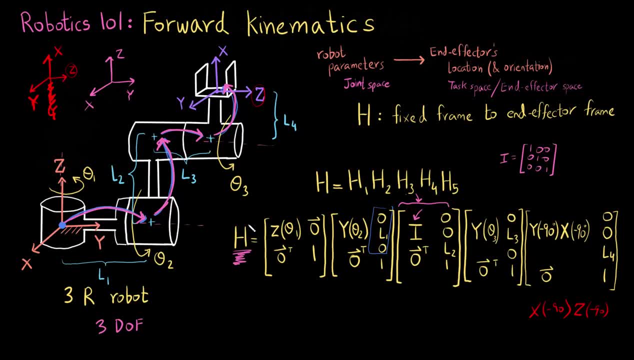 is always going to be the same. it doesn't matter what steps you take to get to that. you can like do the way that i did by using five homogeneous. you can even get clever and you can you do using four homogeneous transformations. uh, you can do six homogeneous transformations, however many you. 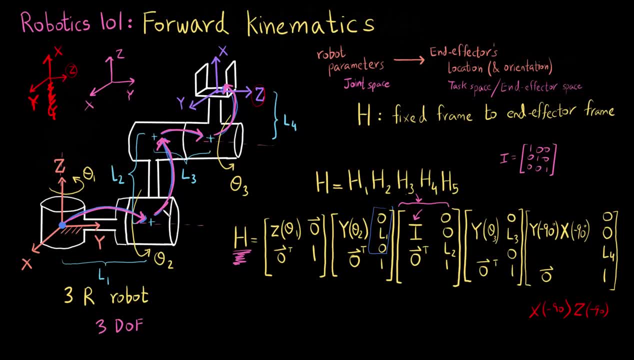 like. however, once you multiply all of them out, the homogeneous transformation that you are going to get at the end is going to be the same. so one way that you can do it is probably like you can combine the these two homogeneous transforms into one. so what you can say is: if you, if you are. 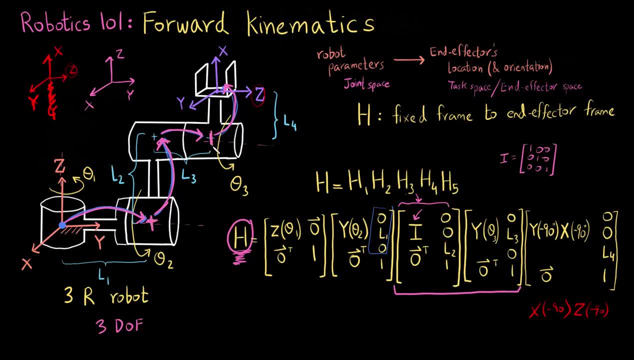 if you have your uh frame here and you want to go here. so what you would do is you would uh first displace it along the y-axis by a3 and z-axis by 82 and then rotate it, so you can just combine these two together and you can just write uh this: so there is.